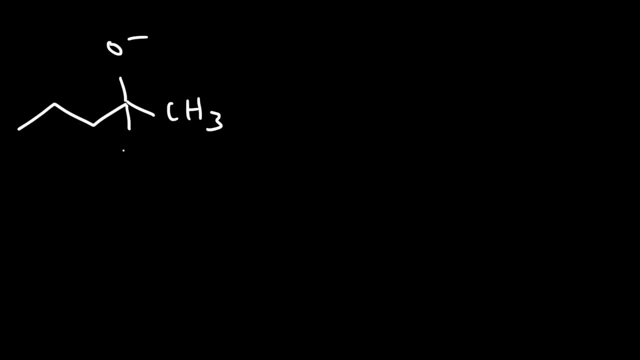 the oxygen with a negative charge is going to receive a proton from the hydronium ion, So it's going to grab a hydrogen, turning into a secondary alcohol, And so this is the major product for this reaction. Now let's work on another example. So here we have cyclopentanone and let's react it with. 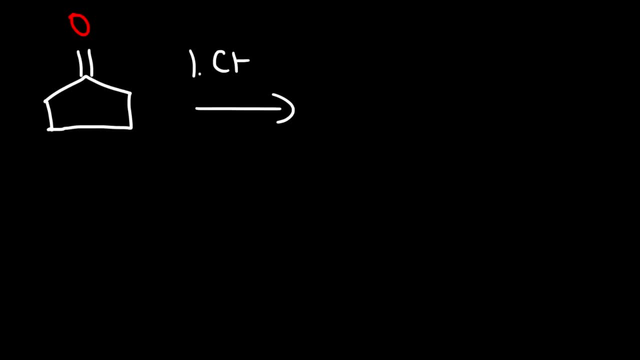 we'll use the same. actually, let's use a different reagent, This time ethyl magnesium bromide. So feel free to pause the video and work on this example So we could follow the same process. So the Grignard reagent will attack the carbonyl carbon from the back. 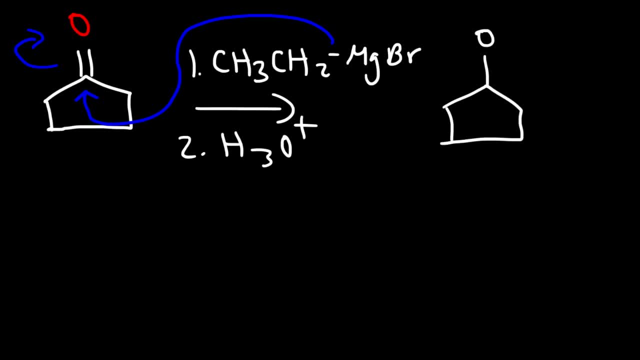 Giving us an alkoxide ion, And here is the ethyl group that we've added to it. Now, in the next step, it's going to pick up a hydrogen, And so this is going to give us a tertiary alcohol this time, And so this 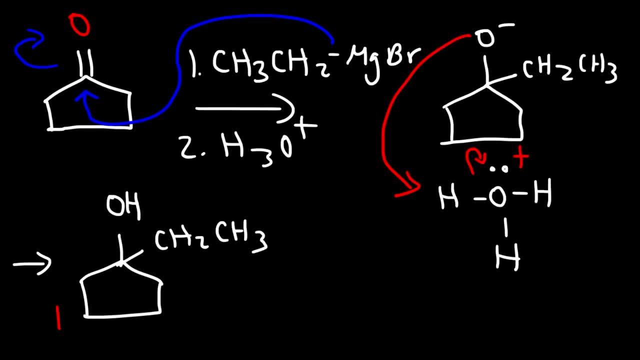 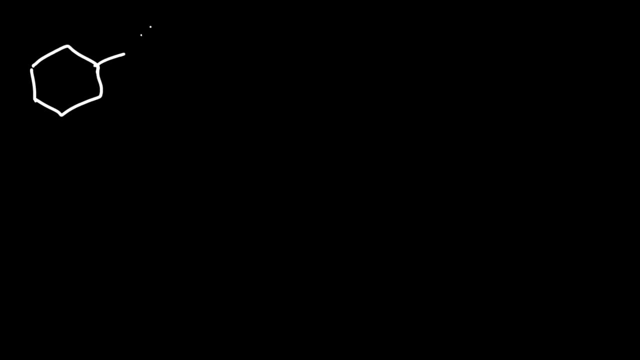 is the major product for the reaction. So anytime you mix a Grignard reagent with a ketone, you're going to get a tertiary alcohol. So now let's move on to our next example. So here we have bromobenzene, And in the first step we're 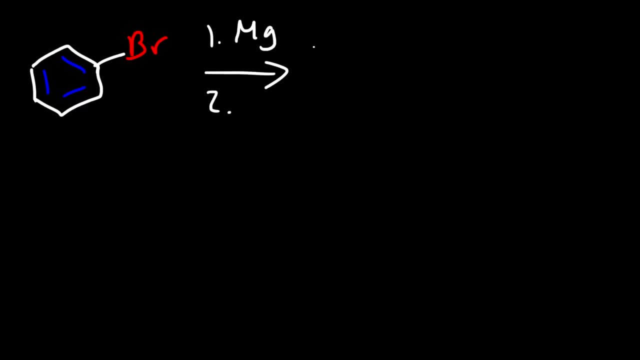 going to react it with magnesium And then, in the second step, carbon dioxide And then in the third step, H2O+. So feel free to pause the video and work on this problem. So once we add magnesium to bromobenzene, magnesium will insert itself between 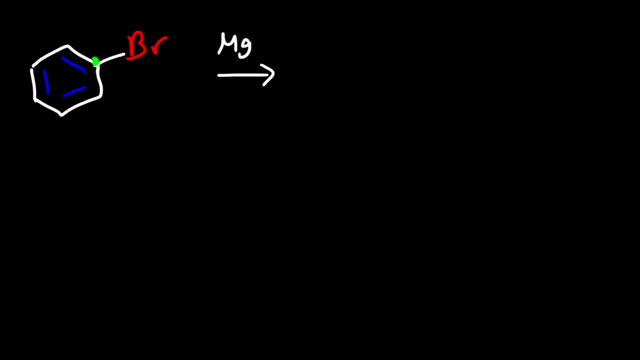 this carbon atom and this bromine atom, And so this is going to give us phenyl magnesium bromide. Now, in the next step, il's going to react with carbon dioxide. So this carbon is partially positive, but the carbon attached to the 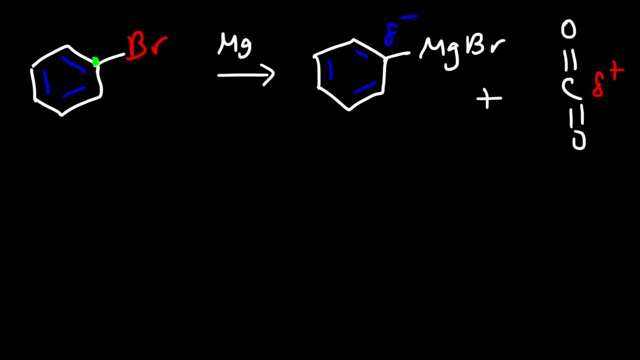 magnesium atom. that carbon is partially negative And so it's going to attack this carbon, breaking the one of its pi bonds. Mule: increase kinds of auststanbul hope. Mule: increase kinds of aust pean. Mule increase kinds of aust Bros Jessie Mule increase kinds of aust factualผม. 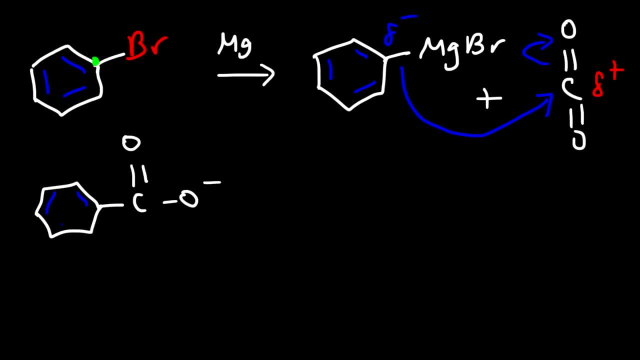 And now we have benzoate. We also have the magnesium ion in the solution with the bromide ion. So if you want to, you could write this like this: You could attach the oxygen with the negative charge to MgBr if you want to, but I'm not. 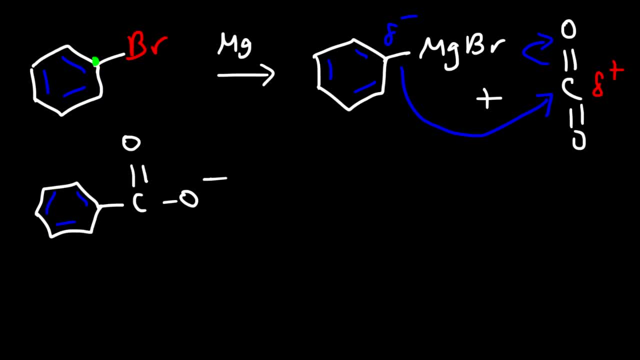 going to worry about the magnesium and the bromine atom at this time. So the last step is to react it with H2O+, And so the final product for this reaction is benzoic acid. Now let's move on to our next example. 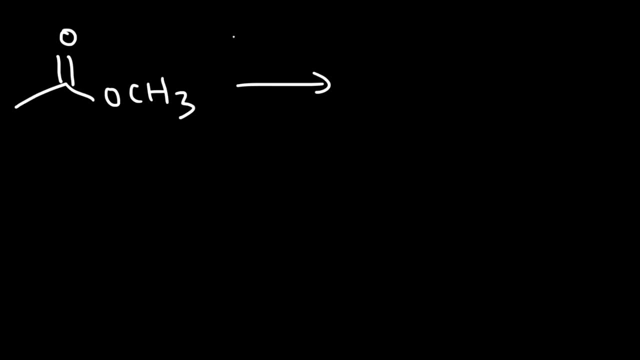 So what happens if we make a reaction? We're going to mix an ester with a Grignard reagent, So we're going to react it with ethyl magnesium bromide, followed by H2O+. Now, when reacting a Grignard reagent with an aldehyde or ketone, you can only add one. 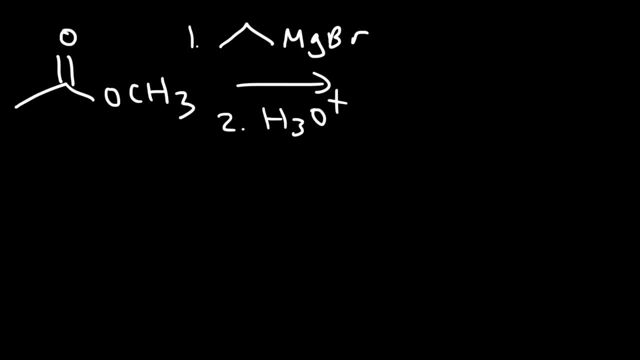 R group. But with esters and acid chlorides you can add two R groups. So in this example you'll see that we're going to add two ethyl groups to the ester. So let's go ahead and begin. So this is going to be the first nucleophilic addition. 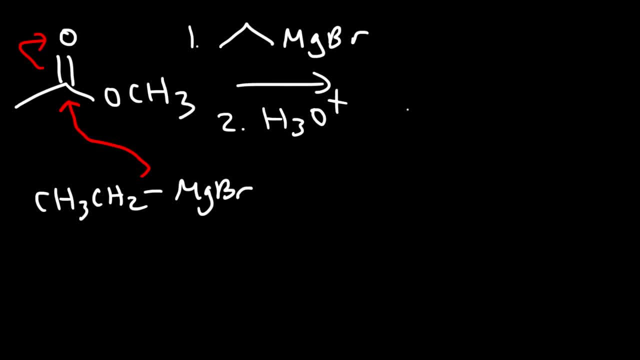 Ethyl magnesium bromide will attack the carbonyl carbon, giving us a tetrahedral intermediate, And so here's the ethyl group that we've added at this point. That's the first R group. Now we do have a relatively decent leaving group compared to this group. So we can kick out the methoxide ion And thus we're going to get a ketone. Now this same Grignard reagent can react with a ketone, So it's going to attack the carbonyl carbon, giving us an alkoxide ion. 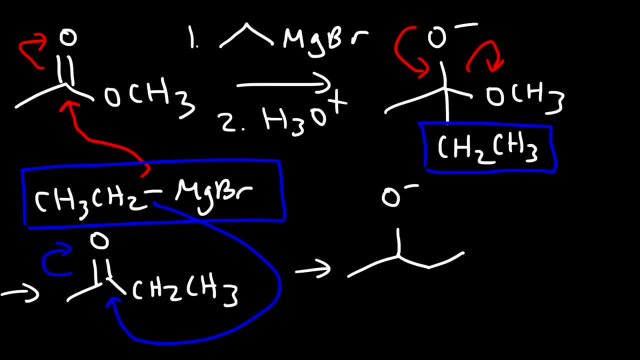 So here is the second R group, But I'm going to write it out for this problem. So this is CaO2.. This is CH2CH3.. And here we have another one. So now the last step is to react this with H3O, plus turning this into an alcohol. 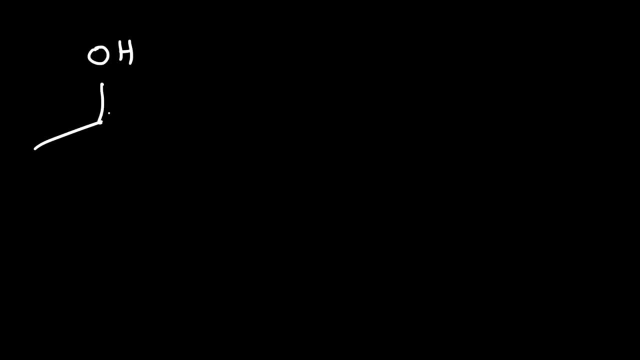 So what we have is a tertiary alcohol. So this is a tertiary alcohol. Now what we do have is a segment of peak alcohol, But this is gonna react with H3Oенная and the ring is gonna react with H3O. So it reacts with H3O because it's going to. 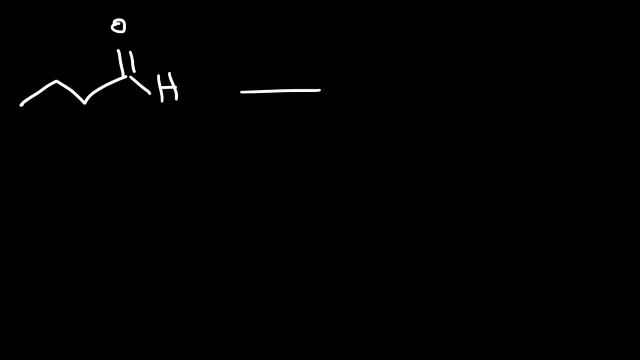 react with H3O- here on the边xi- and with the LFTR. So it reacts with LFTR for about every single territorial molecule that's there, And so this is the major product for the reaction. As you can see, the Grignard reagent reacts twice with the ester. 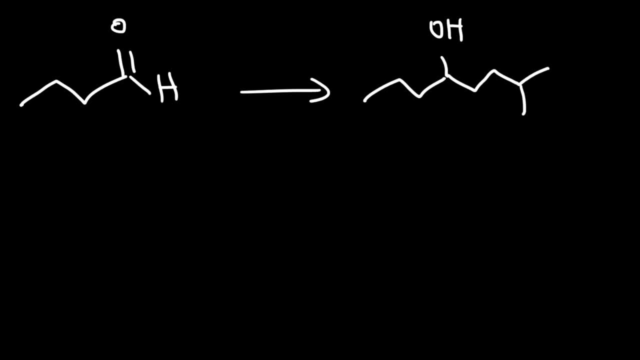 It adds two R groups to it. Now, sometimes you may be given the reactant and a product of a reaction And you need to determine the reagent that's needed to convert the reactant into the product. However, at various points that we do, we'll get atravate room, and so this will be very echtious. 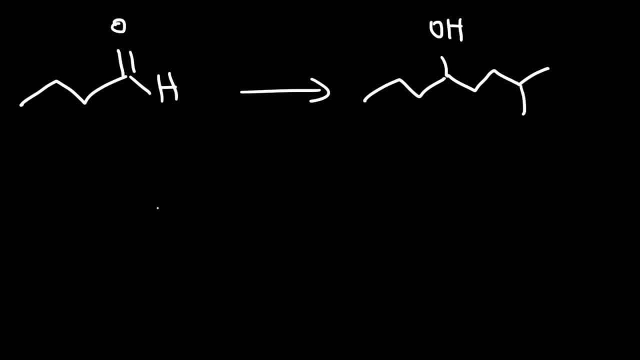 the product, which is what we have in this example. So what do we need in order to make this compound? So we're turning the aldehyde into a secondary alcohol And notice that these four carbons were already present, And so what we added were these carbons. 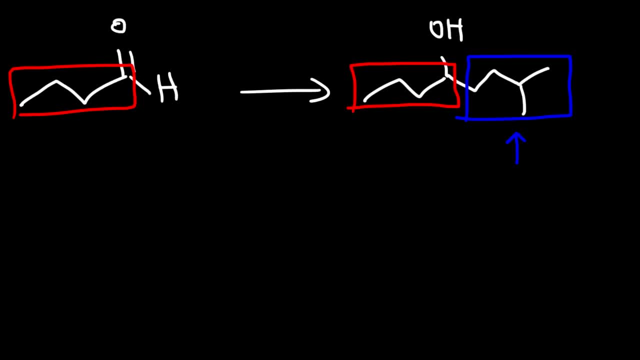 So our green reagent will need to contain this group. So basically, on this carbon, you need to add the green reagent, And so basically all I did was draw what I saw right there and just add MgBr to that carbon atom. So that's going to be the first step. And remember when converting the aldehyde: 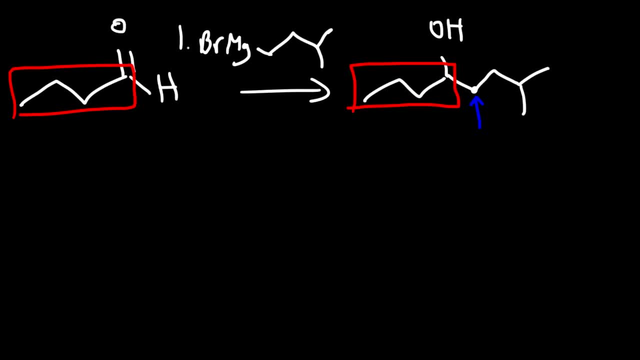 into an alcohol. you only need to add the green reagent once, So we only need one equivalent of MgBr Of this green reagent, And then, in the second step, we simply need to use H2O+, And so that's. 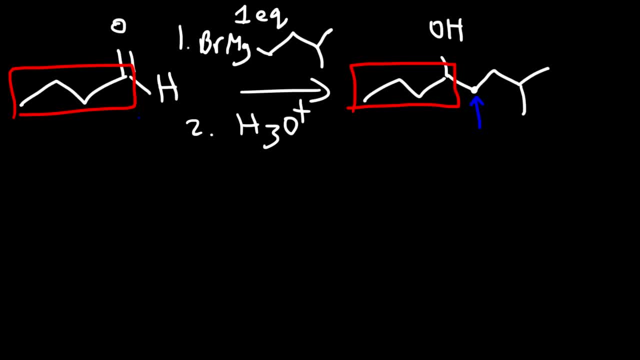 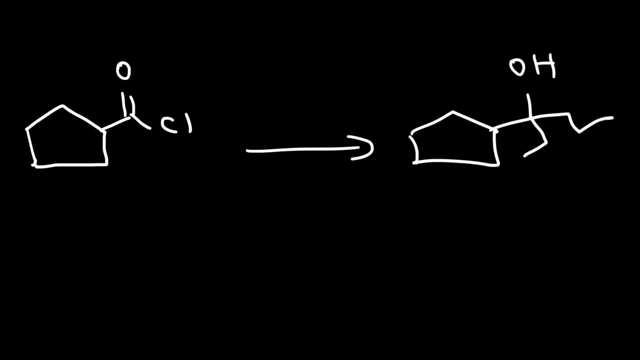 how you can determine the reagents that you need in order to go from this aldehyde into this secondary alcohol. Now let's work on another example. So here we have an acid chloride and we wish to convert it to a tertiary alcohol. What reagents do we need? So we already have these six carbons. 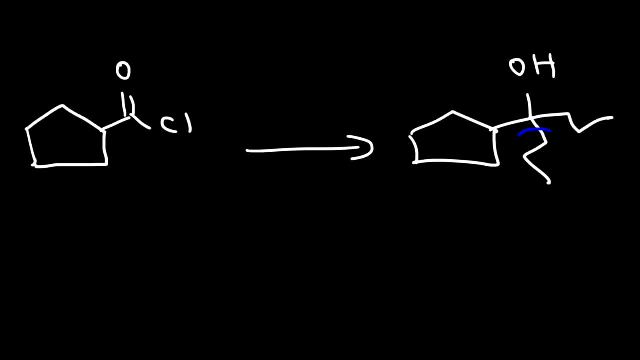 What we need to add are these two propyl groups, And recall that when mixing a green reagent with an acid chloride or an ester, two R groups will be added, And those two R groups are the same. We need to add two propyl groups. 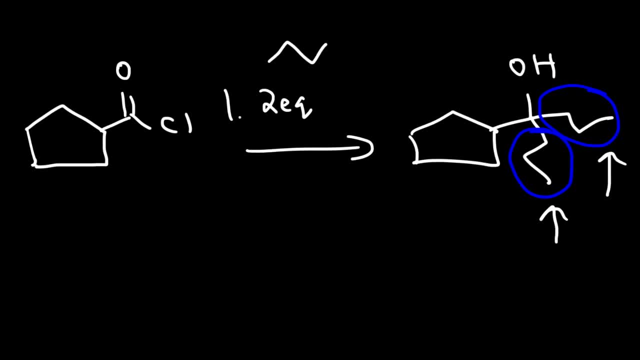 So in step one, I need to add two propyl groups. I need two equivalents of propyl magnesium bromide, And then, in step two, just H2O+. That's all we need to do Now. the mechanism by which the green reagent reacts with an. 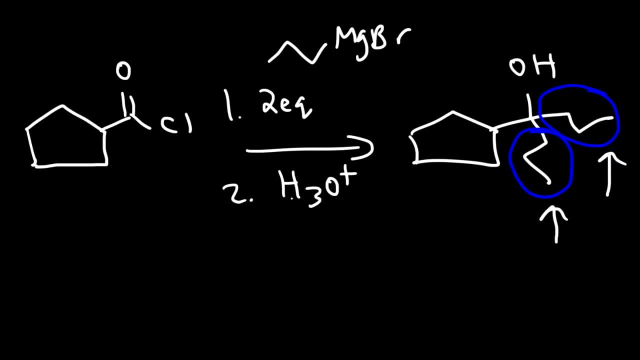 acid chloride is virtually the same when it reacts with an ester. The only difference is, instead of having an OCH3 group, you have a Cl group, which is the better leaving group. Go ahead and try this problem. Let's say we have one group of OCH3. And we need to add. 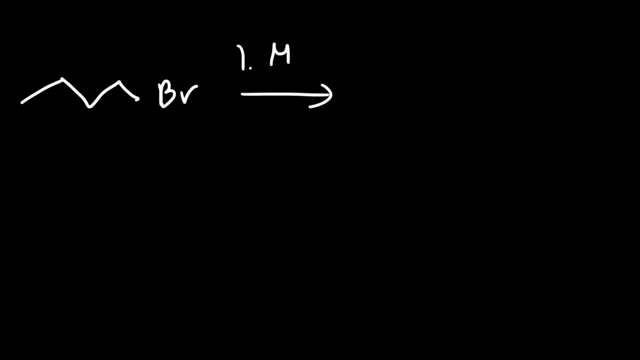 one bromobutane, And in the first step we're going to react with magnesium, And then, in the second step, ethylene oxide And then H2O+ in the third step. What is the major product of that reaction? 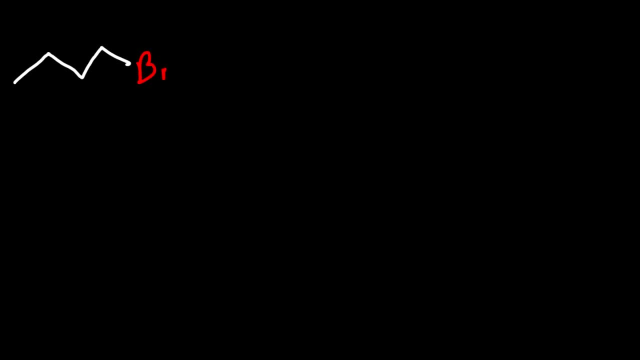 So let's take this one step at a time. So let's take butyl bromide and let's react it with magnesium. So this is going to give us butylmagnesium, And then, in the next step, we're going to react that with ethylene oxide, And so the 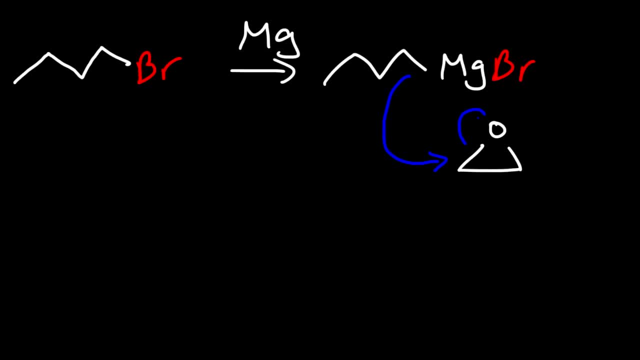 green reagent will attack one of these carbons. Because it's symmetrical, it doesn't really matter which side we attack. So we're going to add two carbons to our four carbon chain, So we're going to have a total of six carbons, And so on. the last carbon, that carbon is